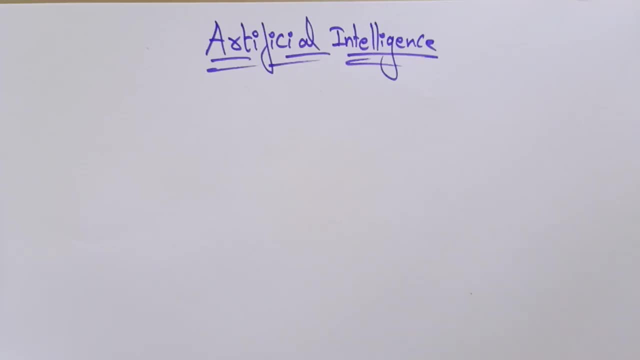 Hi students, welcome back. So now coming to the next subject: artificial intelligence. So, artificial intelligence, This is a very important subject in the computer science environments because nowadays we are all leading dealing with this artificial intelligence. Today's technology is growing very fast and we are getting in touch with different new technologies day by day. Okay, so this artificial intelligence is one of the five. 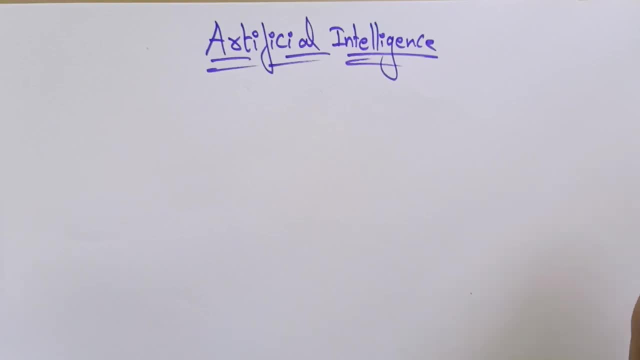 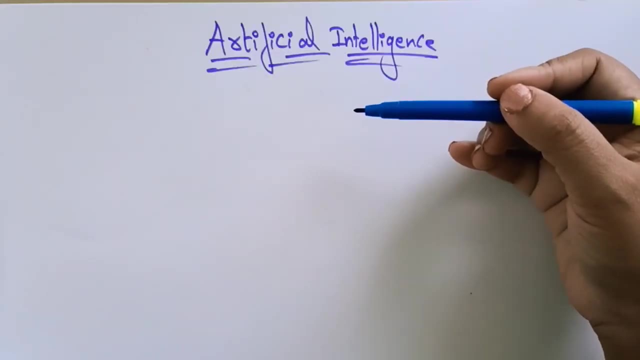 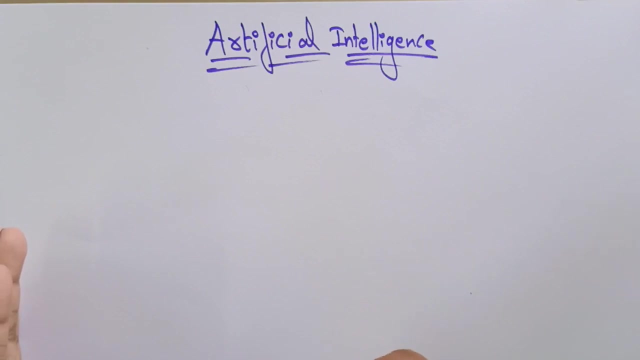 fascinating and universal field of computer science which has a greatest scope in the future. Okay, and it has a tendency to cause a machine to work as a human. That is a main concept. The machine has to work as a human because of this artificial intelligence. Okay, so at present, artificial intelligence, currently working with a variety of subfields, means whatever you're dealing nowadays- so many technologies, so many gadgets that you're. 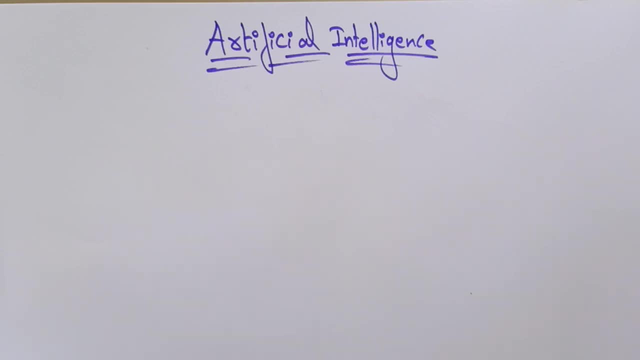 using. it's completely based on the artificial intelligence like, ranging from general to specific, Like, if you take the self driving cars, Nowadays, this is a most important and the most efficiently used as a self driving car. Okay, and playing chess in your mobile phones: it is using the technology of artificial intelligence. and playing music, painting everything. it's that relating to this artificial intelligence, Okay, so that's why I'm saying this is very 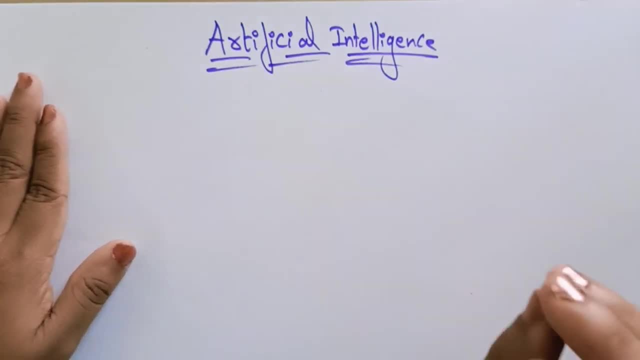 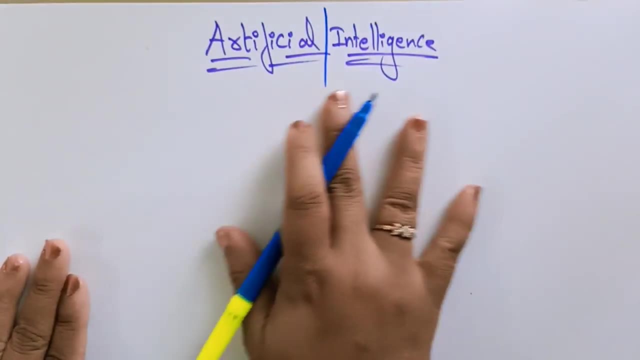 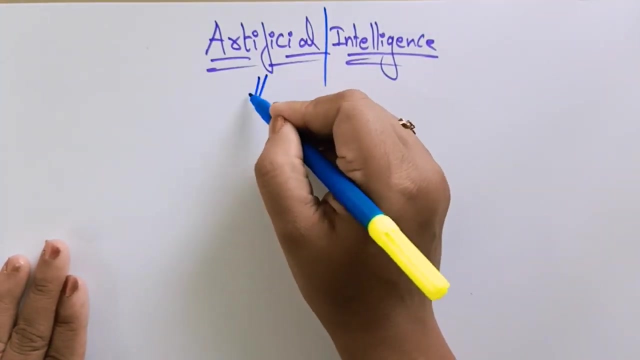 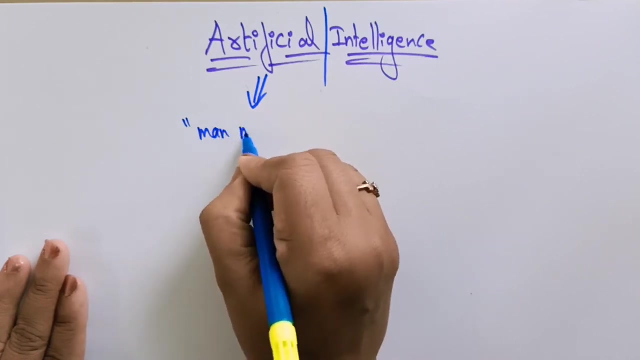 important subject and important concept in the computer science environment. So first let's see what is this artificial intelligence? I'm breaking this word, a single word, into two words. One is artificial and another is intelligence Artificial. What is this artificial? Okay, this artificial defines manmade. The manmade things are artificial. So this pen, it's artificial, Okay, whatever. 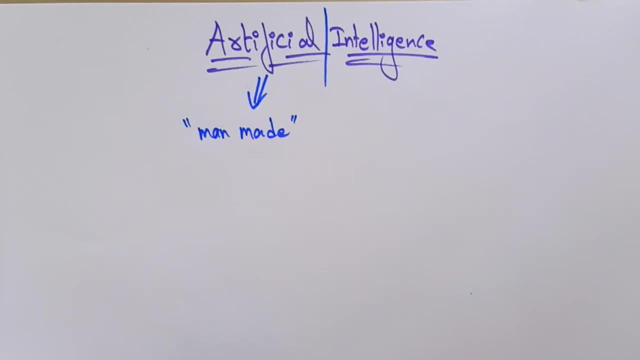 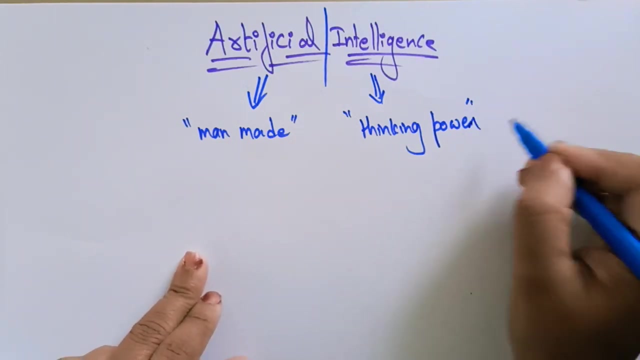 it is not the manmade things are. all comes under the artificial. Then what about the intelligence? Intelligence defines thinking power. Thinking power, So manmade thinking power. you call it as an artificial intelligence. So if you just clap this, artificial intelligence means manmade thinking power. Okay, so whatever the man is going to design that. 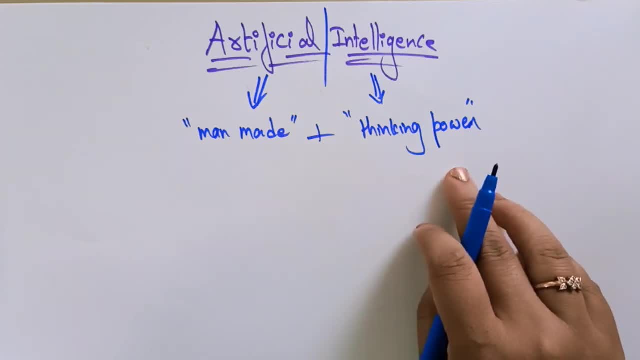 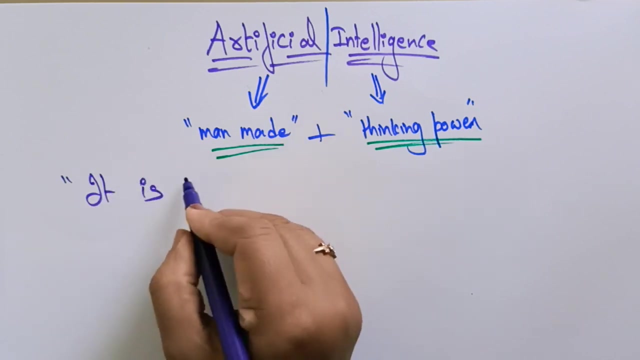 gadget or that thing is having a thinking power. If that system is having a thinking power, then you can say that is an artificial intelligence. So hence, what is the definition of artificial intelligence? Actually, AI means manmade thinking power. Okay, it's a manmade thinking power. So artificial intelligence is defined. as I'm writing the definition, It is a branch of computer science, It's just a branch of. 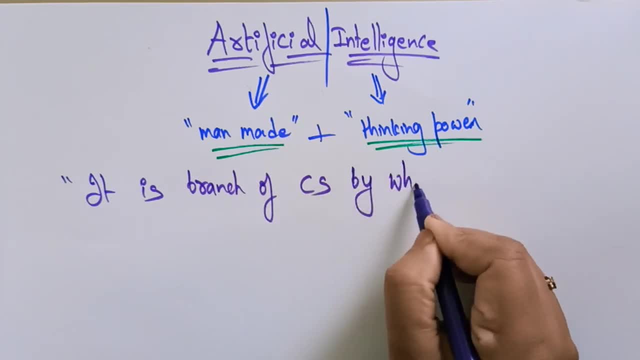 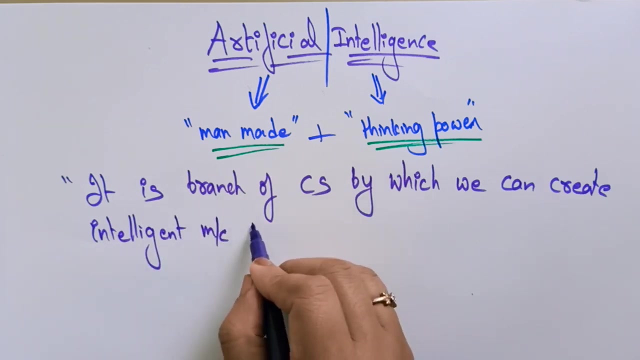 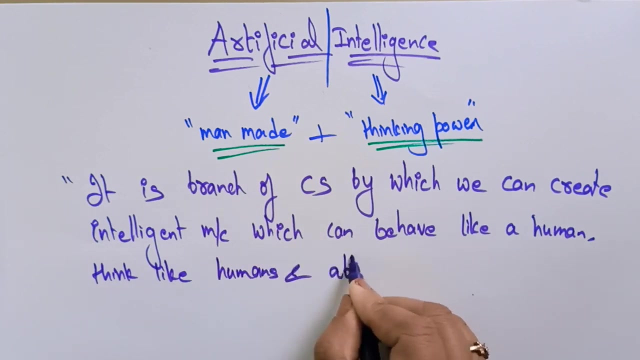 computer science, by which, by which we can create, we can create intelligent machine. We can create an intelligent machine which can behave like a human, which can behave like a human. Not only that, it can think like humans and able to make decisions. also Think like humans and able to make decisions, So that you call it as an. 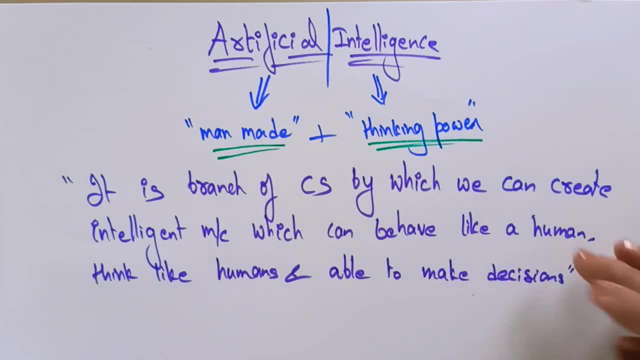 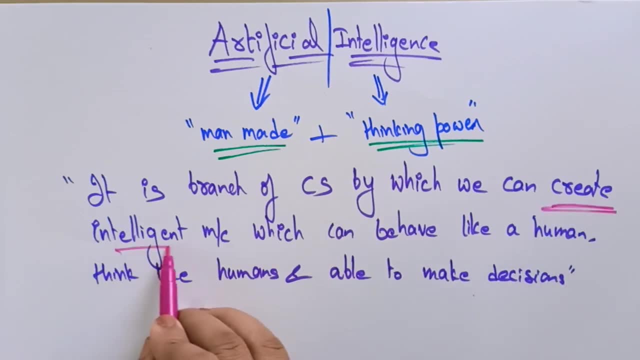 artificial intelligence. So the artificial intelligence is nothing bad. It is a manmade thinking power. It is a branch of computer science by which we can create. we are going to create an intelligent machine, So that machine behaves like a human And also it thinks like a human. 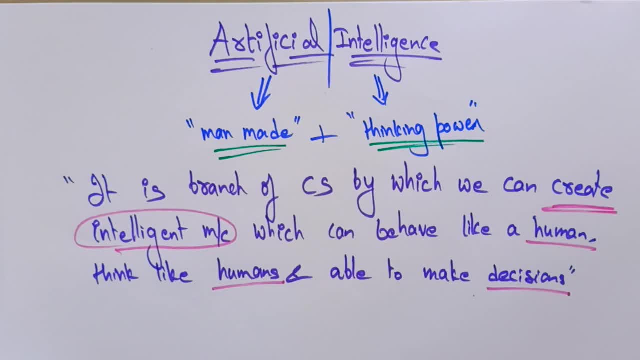 and it also able to take decisions. that you call it as an artificial intelligence. okay, so with artificial intelligence you do not need to pre-program a machine to do some work. so far what you have seen. so if you take your mobile phone means, suppose, if you are taking any gadget. 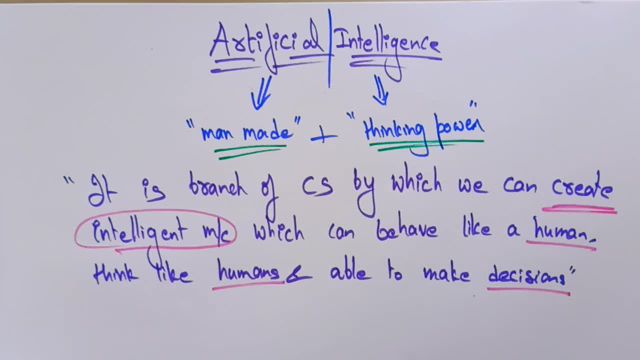 electronic gadget, so that gadget is already programmed, pre-programmed, a machine to do some work. if you are taking a televisions, if you are taking a computer, whatever you are taking, so at simple thing, that is pre-programmed, everything is pre-programmed. so this mobile phone is just. 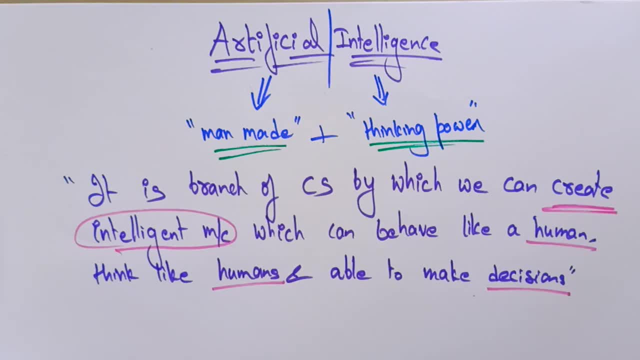 pre-programmed to make to receive the calls. if you take the normal gadget, it's just a pre-programmed to receive the calls and to access to make the calls, okay. so despite that, you can create a machine with programmed algorithm which can work with own intelligence, and that is the awesomeness. 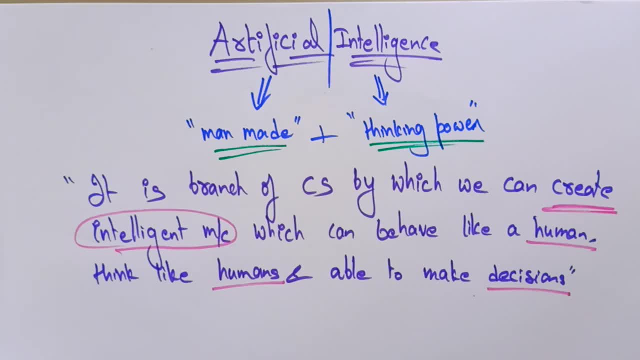 awesomeness of the artificial intelligence. okay, okay, let me let me explain you again. so with artificial artificial intelligence- you let me write that point- with artificial intelligence, you do not need to pre-program. so this is an important thing, you do not? you do not need to pre-program the machine. 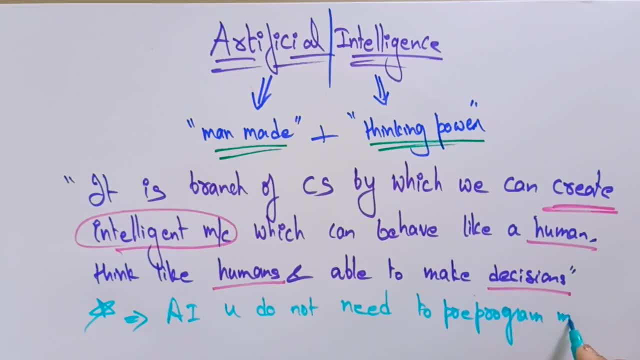 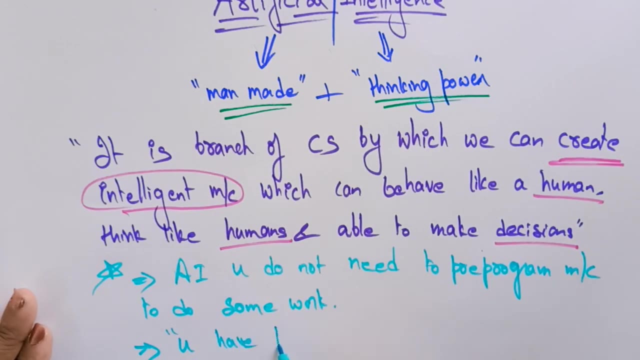 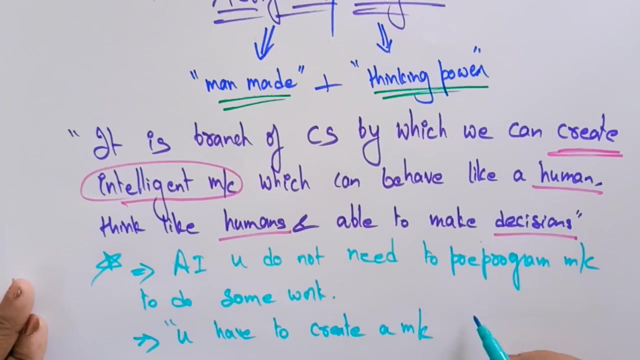 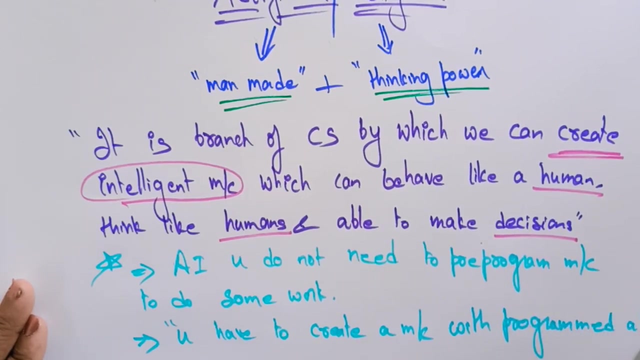 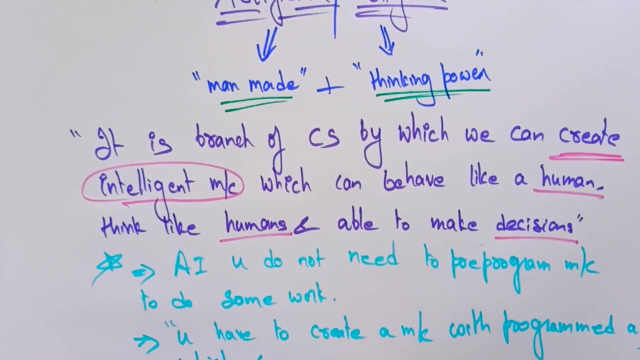 pre-program machine to do some work. to do some work. so, despite that, you can create a machine with programmed algorithm. so you have to create a. you have to create a machine with what, with what? you have to create a machine with programmed algorithm, with programmed algorithm which can work with own intelligence. that is a main point which can work. 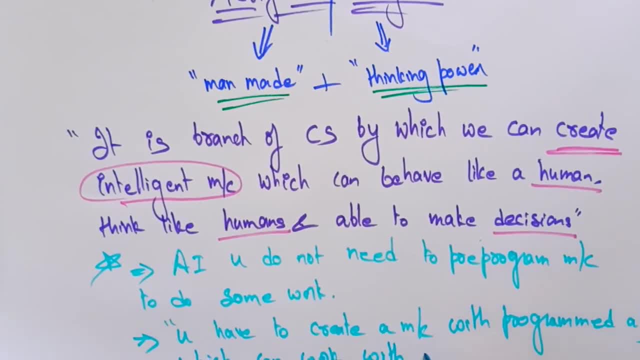 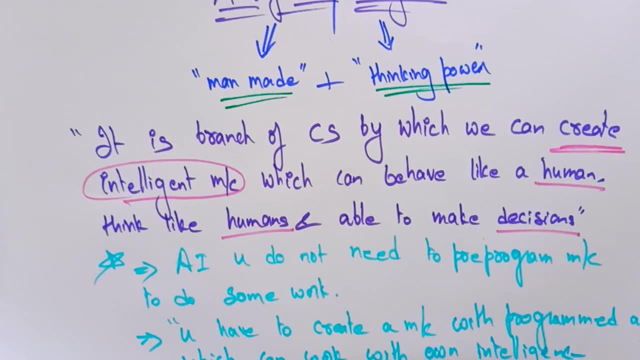 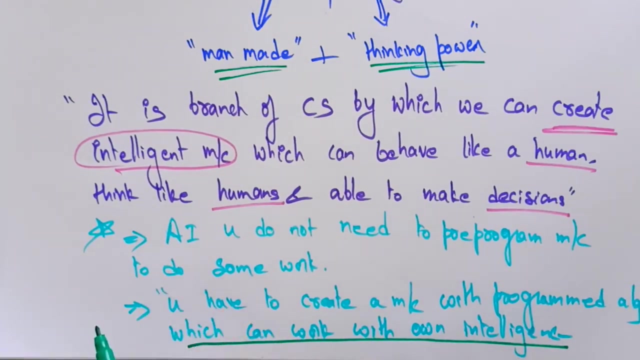 with own intelligence. so that program you are designing, so you are going to design a program which can work with own intelligence. so that is it. so in a, a artificial intelligence, do not need a pre-programming machine to do some work. why we don't need it? because if you- uh, it's general. 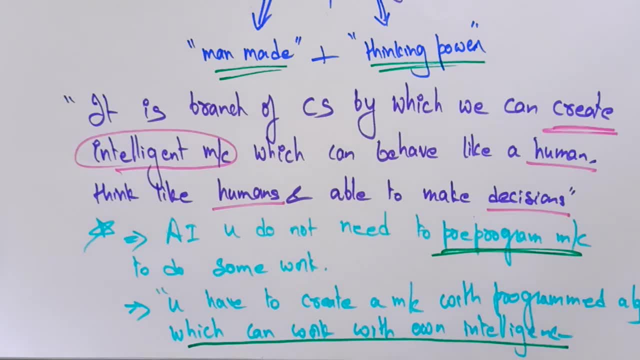 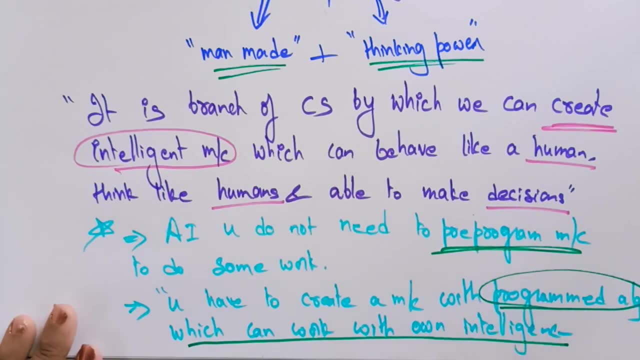 machines. what you are doing, you are just pre-programming and it is only doing that task, particular task. but whereas artificial intelligence, you are going to programmed an algorithm, what type of algorithm you are programming which can work with own intelligence? that program you designed in a way that that program will do its thinking power. okay, it is, it can take its own decisions. 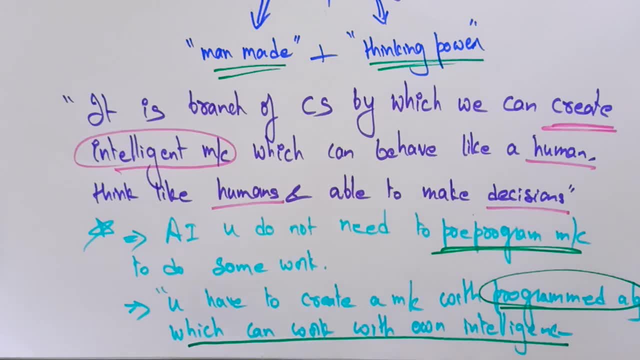 it can work with own intelligence. that type of program you designed that program. you can call it as an artificial intelligence, which is a man-made thinking power. you are creating a program which is a man-made thinking power. you are creating a program which is a man-made thinking power. 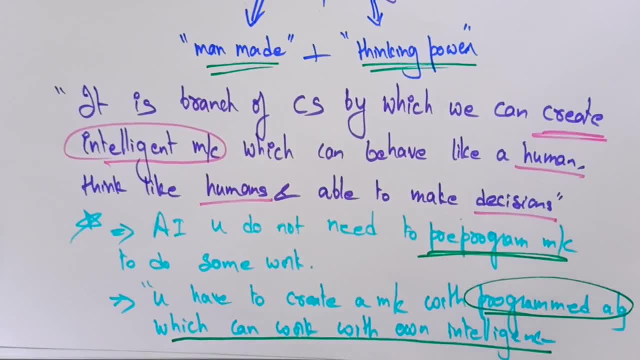 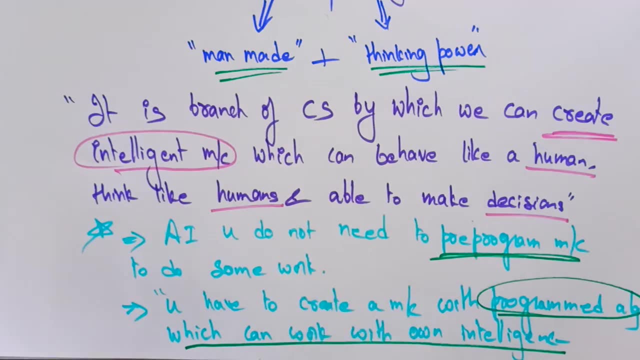 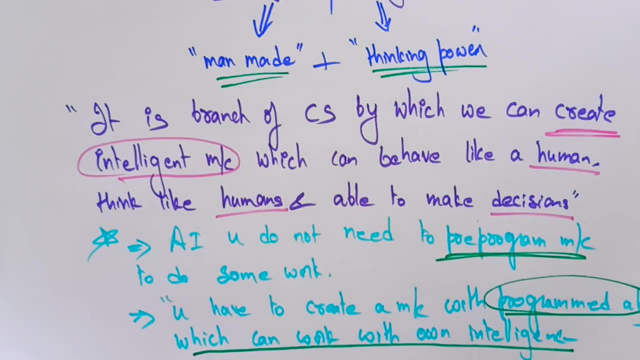 okay, so which is an awesomeness of artificial intelligent, is it clear? so i hope you understand. uh, so i just explained the definition. it is a man-made thinking power. why we are called it as a man-made thinking power? because here we are creating a program, a creating a machine with.